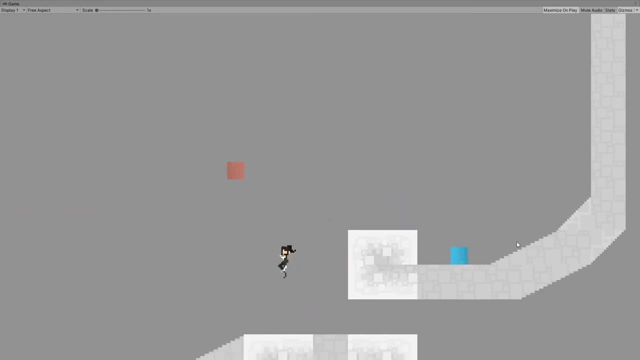 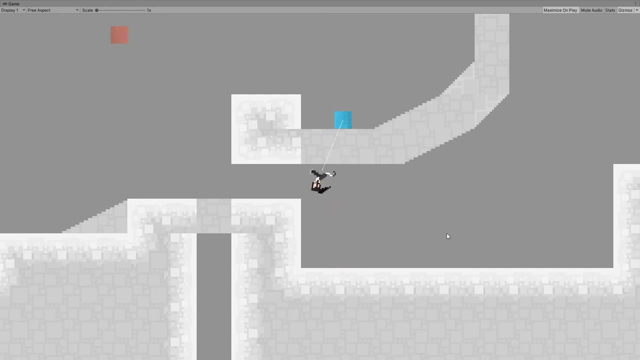 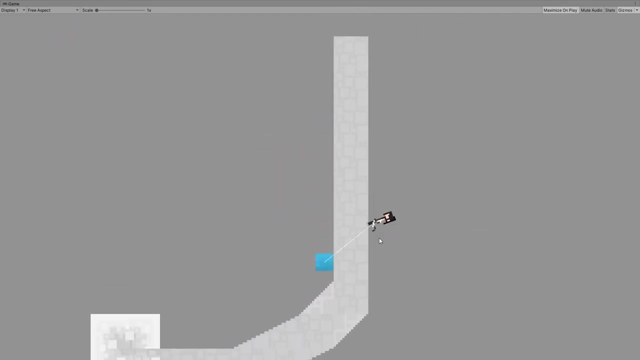 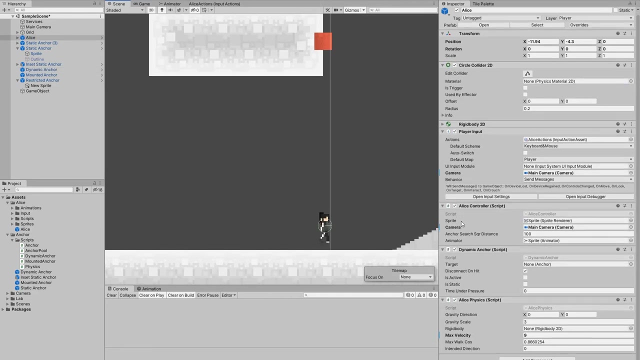 This is also fun. This dynamic anchor can serve as a static one if there's a wall between. Also, I can drag it alongside the wall, which for now looks a little bit broken, but we can make a mechanic out of that. The best part is that every single anchor player included are based on the same components: anchor and physics. 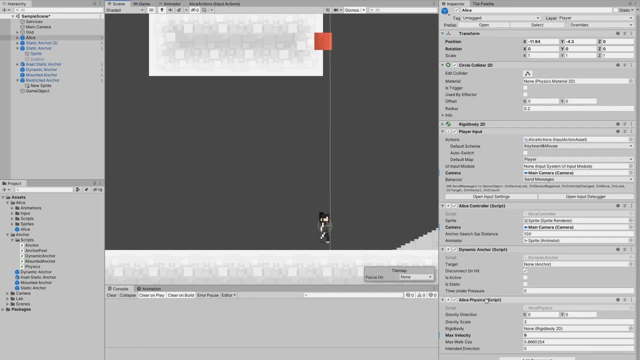